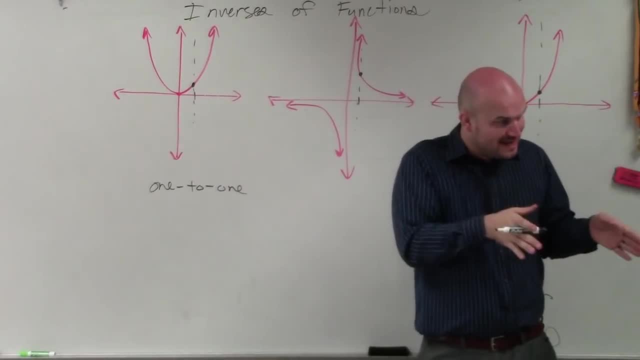 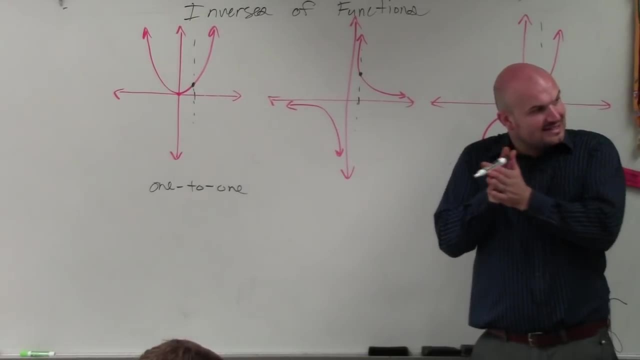 and for every output we're going to have exactly the same input. So the best way to kind of look at that is: for every output you have exactly. so basically you have every input has exactly an output and every output has exactly one input. 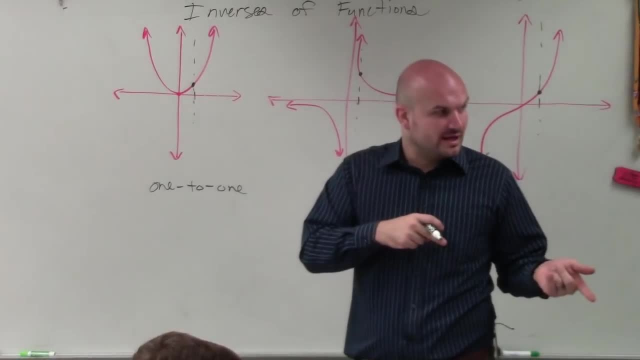 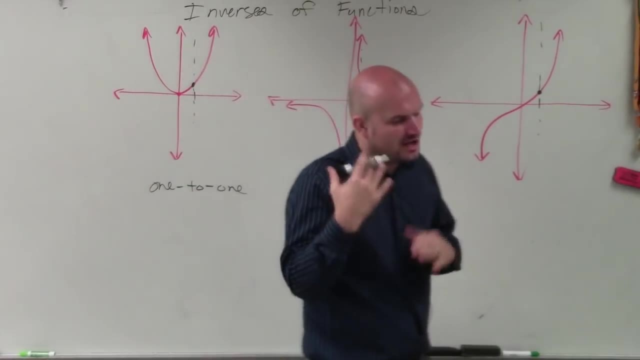 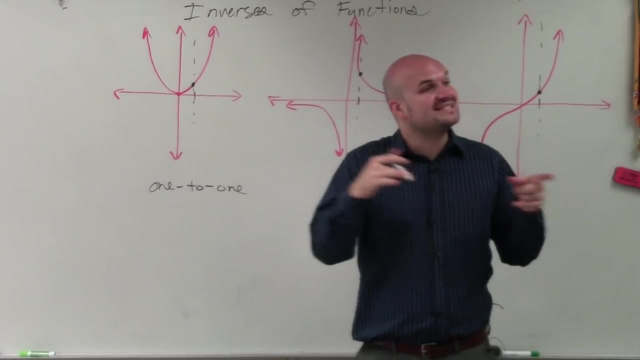 So it's kind of like doing the function test back over again. all right, So I want you guys to understand it. Basically it's uniquely going left and right. Every input has exactly one output, Every output has exactly one input. So remember, if we're determining the function and we said every input had exactly one output, 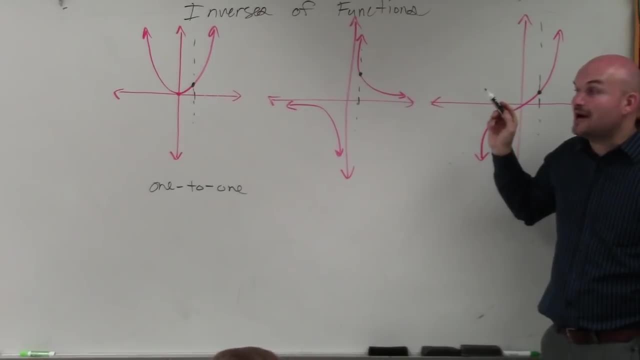 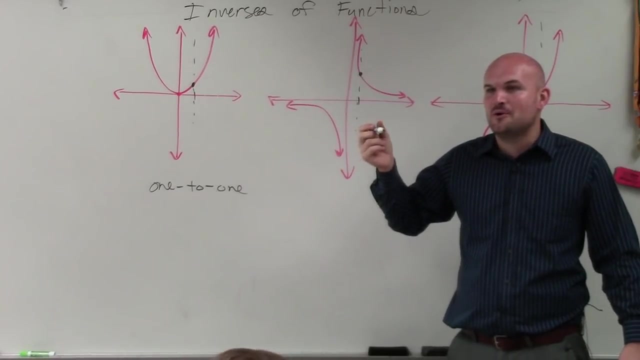 then we use the vertical line test. right Now, if we are going to determine if every output has exactly one input, then we're going to want to use the horizontal line test And basically let's just use 1,, 2,, 3.. Let's go at 3.. 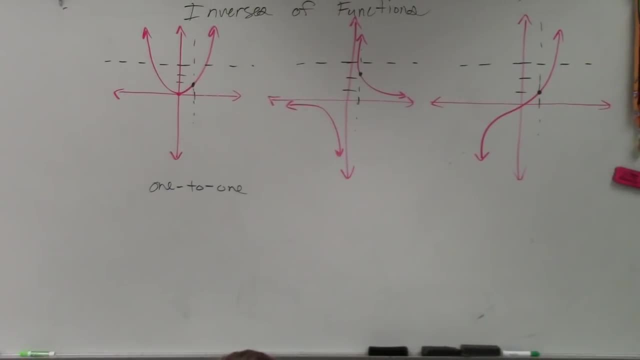 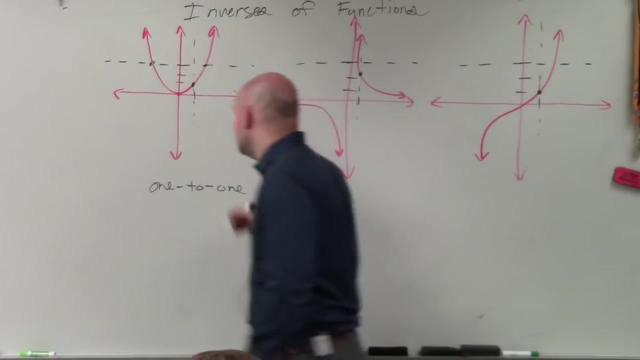 As you guys can see, that when you're doing the horizontal line test, if you have an output that has more than one input, right, that output has more than one input. this example is not 1 to 1.. So what does that matter? Why would we care about if that's not going to have an inverse? 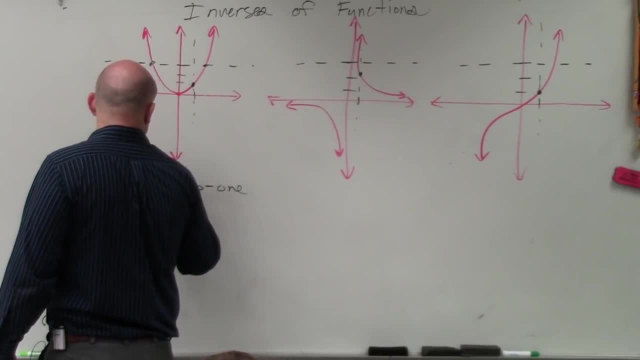 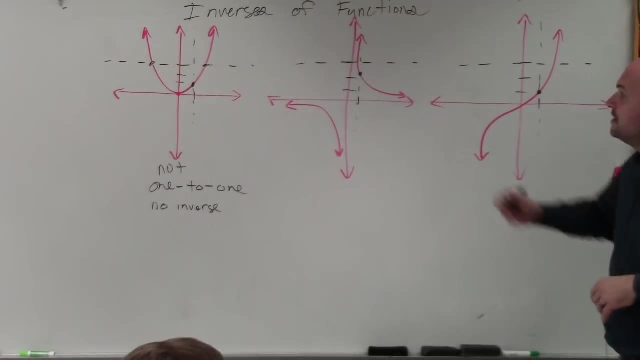 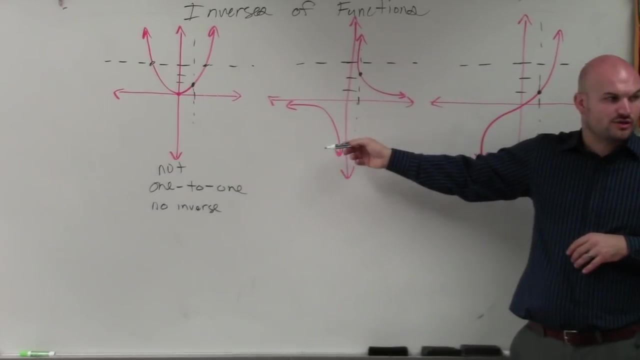 It's not going to have. if it's not 1 to 1, then there's no inverse of the function and I'll explain that in a second. However, this is 1 to 1, right. My one output has one input and there's no other horizontal lines that would cross the. 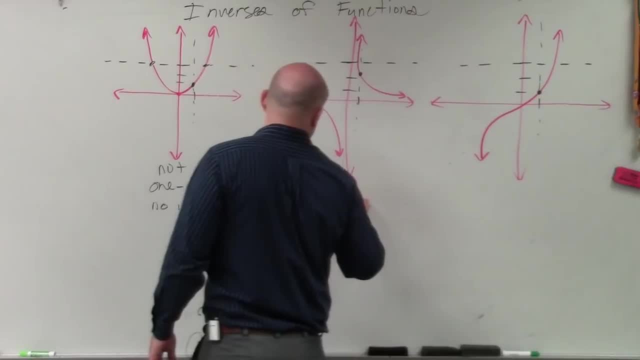 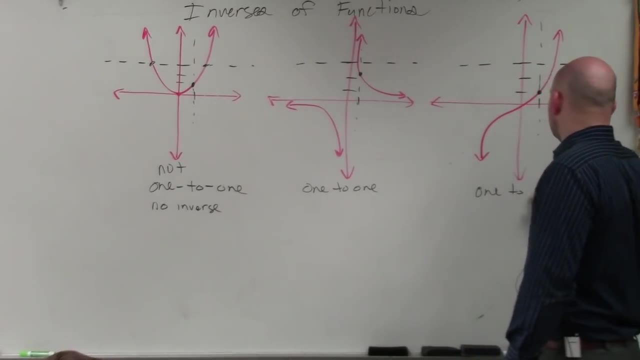 graph more than once, right. So this is what we call 1 to 1.. And this is another example. This is another example of 1 to 1.. So the best way to understand 1 to 1 is basically just using the. 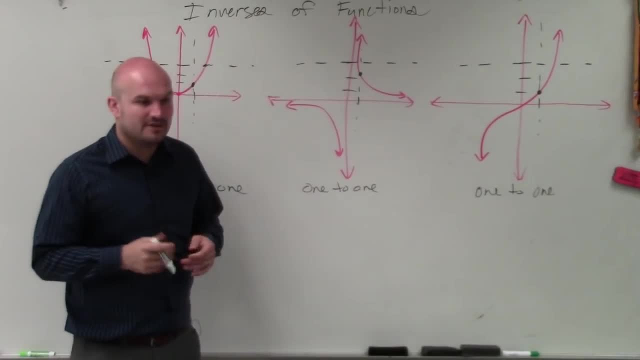 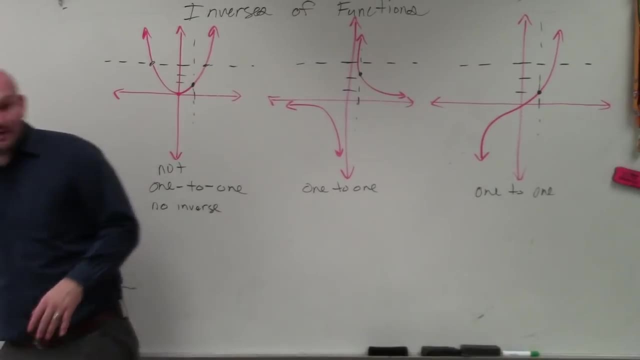 horizontal line test. all right, You guys can write down the definition and I can give it to you, but as long as you guys understand the horizontal line test, that's the most important thing. So what exactly? so now the we know that has an inverse. how can we go ahead and use that to our advantage? 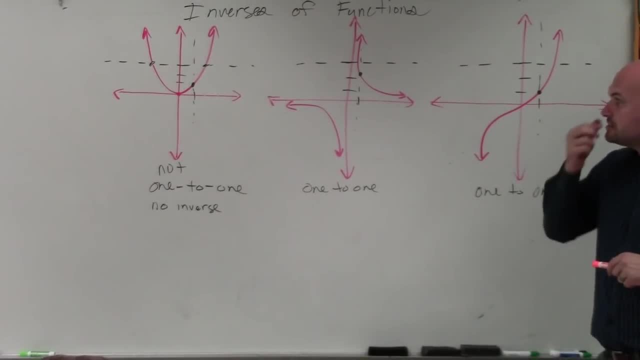 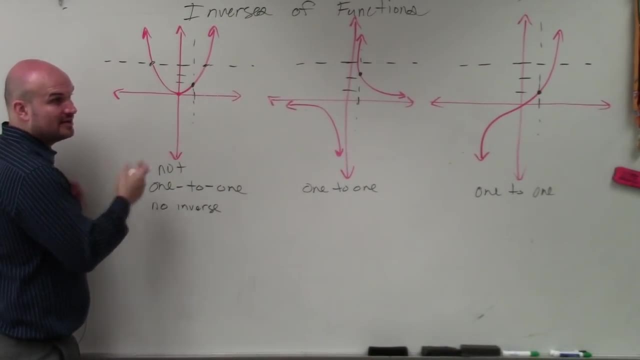 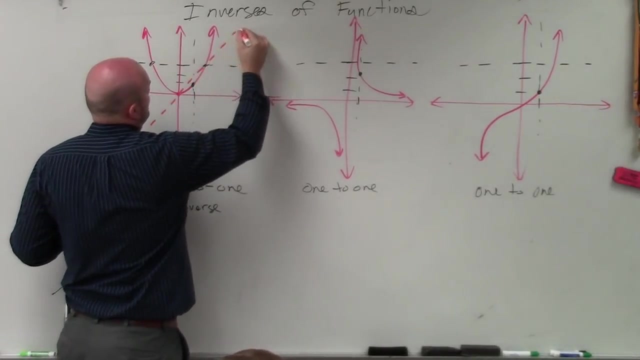 Well, oh, there's my blue. So what we're going to do to graph the inverse. obviously, once you guys learn how to do it algebraically, you can algebraically do it and then plug it in your graphing calculator and graph it. Or if you guys go back to your geometry days, we can get practice. 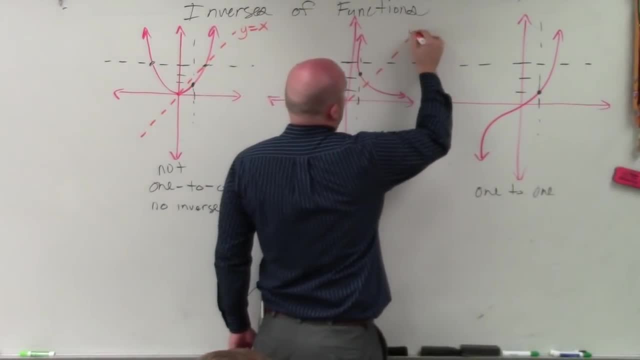 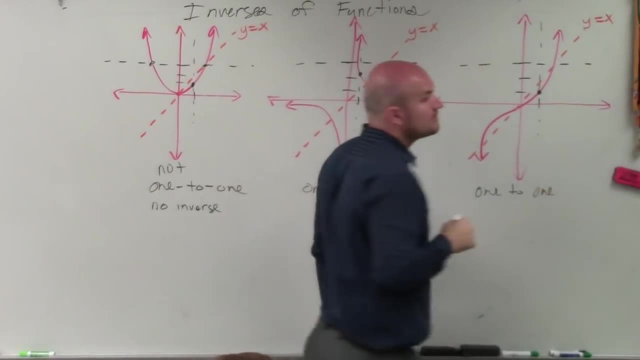 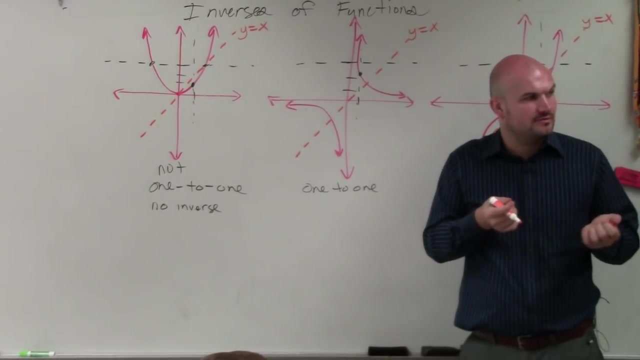 on graphing about the y equals x line. So when you reflect a graph about the y equals x line, you produce the inverse graph. okay, So if you might want to write that down, I'm not going to write it down on this, but by reflecting over, 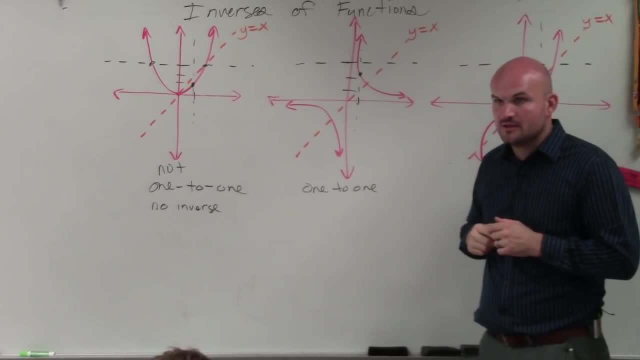 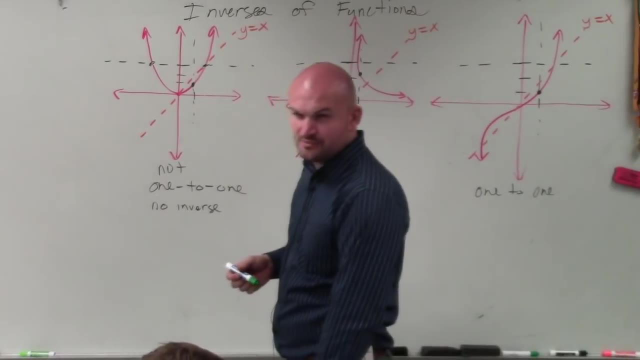 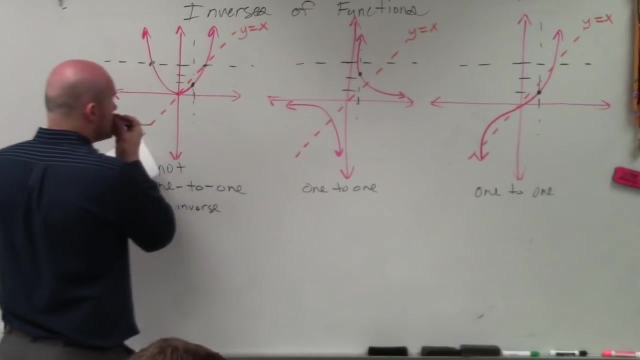 the y equals x line, you produce the inverse function. Now, the best thing I always like to do, that is, whenever you guys are having trouble with reflections, you know, use like a sheet of paper. So if you guys had this graph, you guys can see. 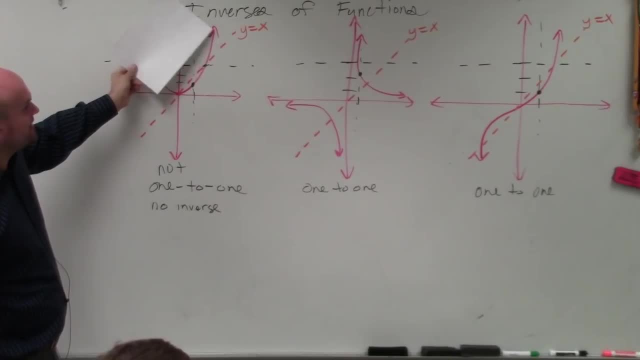 I know what the graph looks like over here. All I'm simply doing is reflecting it over, right. I'm taking whatever is above the line reflected and over Whatever's below the line I'm reflected and above And what you guys would. 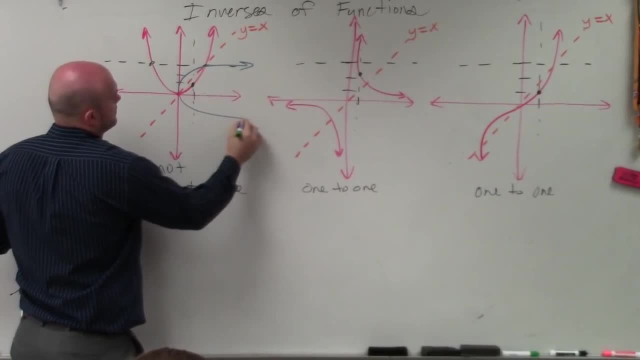 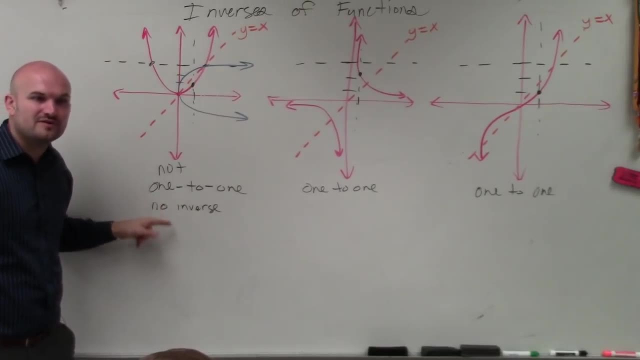 see if you reflected this. the reflection here is not a function, right? Do you guys agree with me? That's why this doesn't have an inverse, that's a function. Do you guys see how the one-to-one property works? When it doesn't pass the horizontal test and you reflect it, it doesn't pass the. 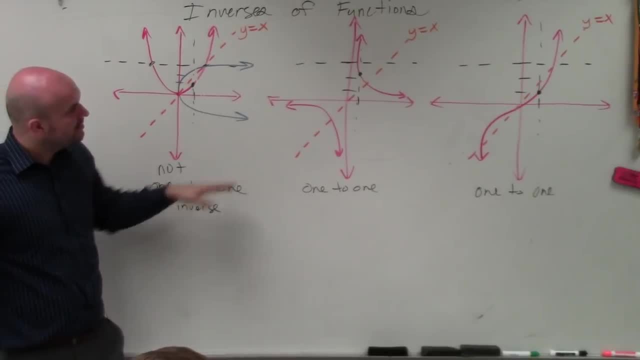 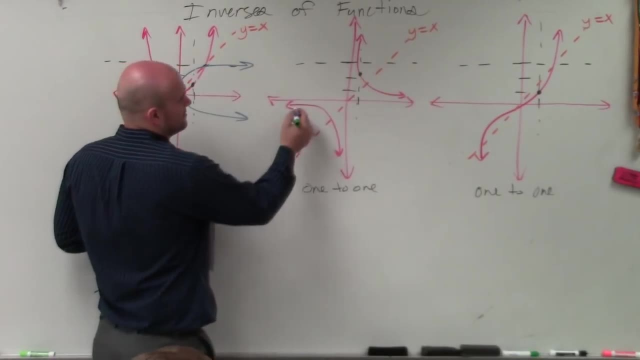 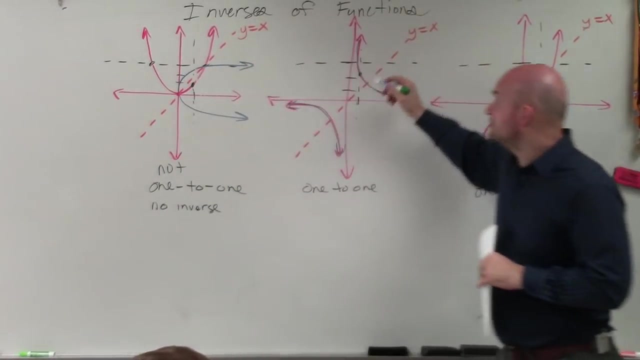 vertical test. That's why we say it doesn't have an inverse Over in this example. this graph is actually reflective about itself. So when I go ahead and reflect about the y equals x, this graph and its inverse is exactly the same. It's an inverse of itself, which is kind of cool. 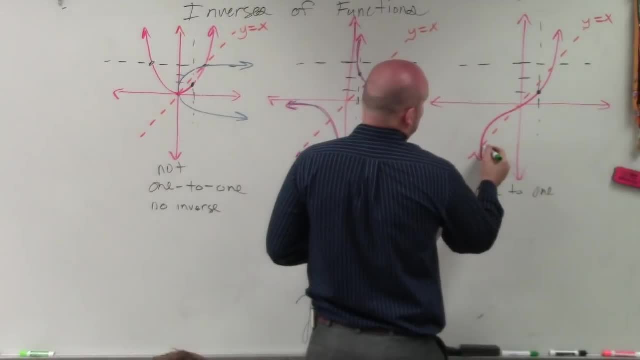 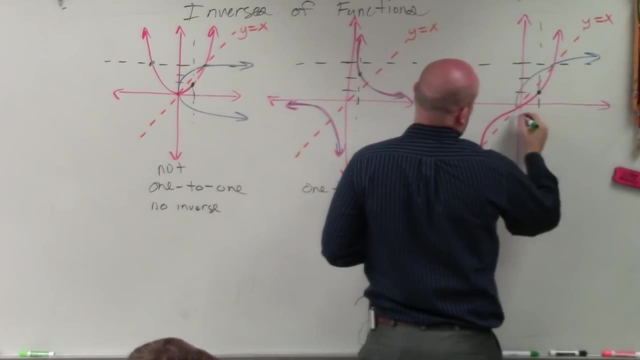 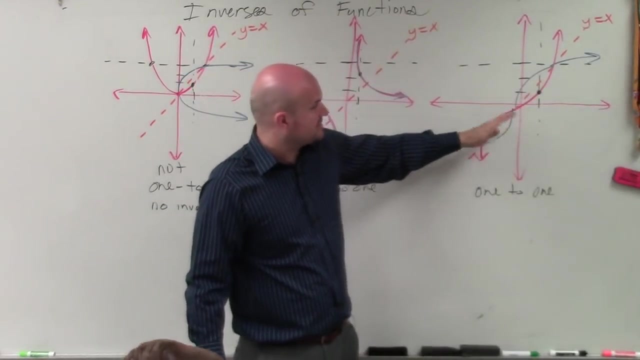 Over here. the graph is going to look something like this. You're basically switching there, And it looks like this, But, again, what you guys can see is that blue graph. What you guys can see, though, is the graph still passes the vertical line test. 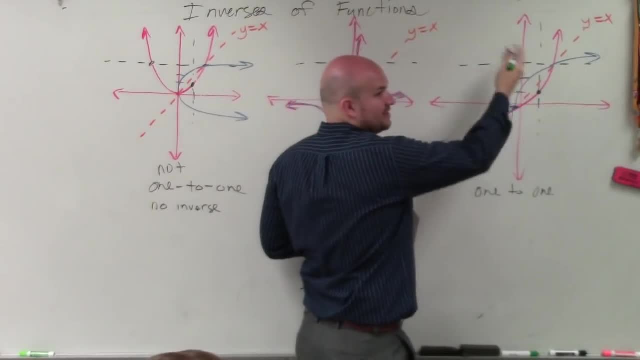 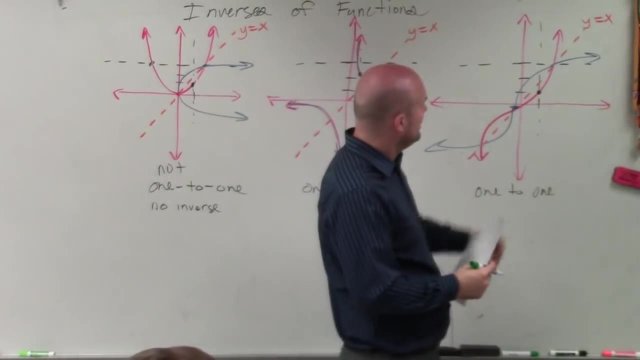 correct. This is just a reflection point, It's not actually two points. So it passes the vertical line test. So that's the blue graph is what's going to be your example. And again, all I did was I took whatever was below the graph. I took whatever was below the graph And I took whatever.